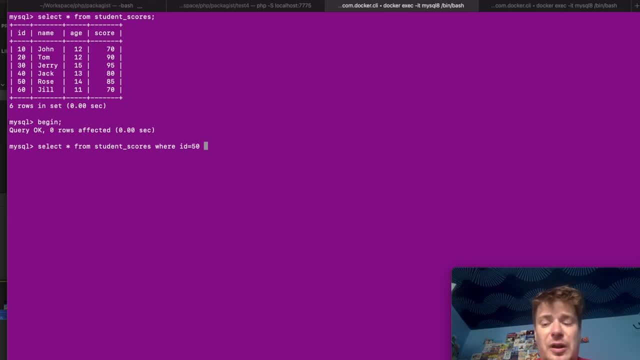 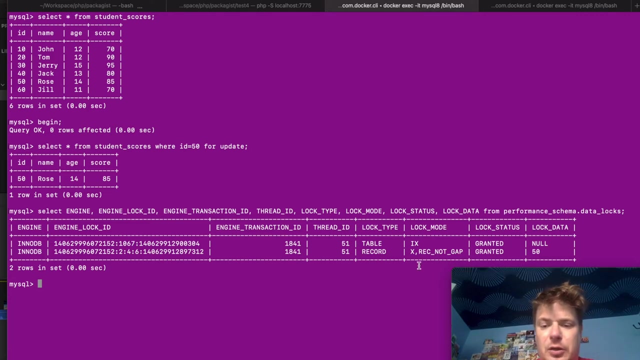 In order to do that, we need to specify the for update keyword in the query. Now the purple session is holding an exclusive lock on one record in the table. We can see this lock by running this query. As you can see, it's actually two locks here, but we are only interested in this one. 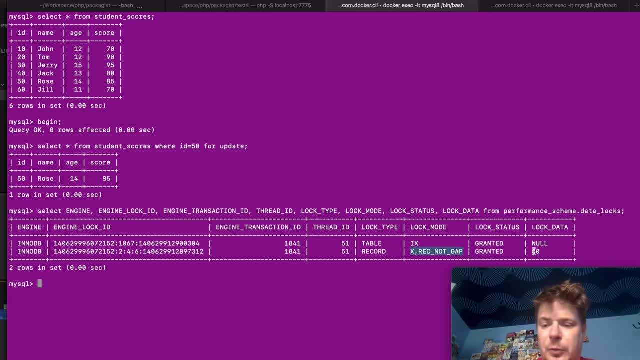 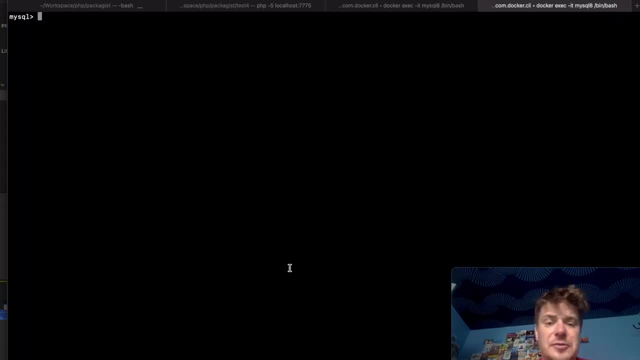 It's an exclusive lock for the record with the ID 50.. So let's jump over to the black session now. We'll start a new transaction here And, like in the purple session, we also want to select one record for update. only this time it will be the record with the ID 60.. 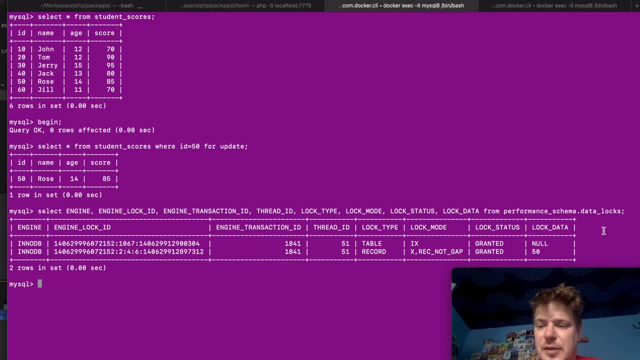 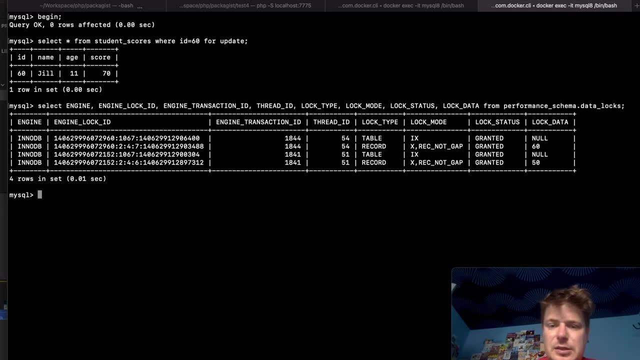 Now let's check what's going on in the locks table. To do that, I'll copy this query and run it here. So, as you can see, we've got two exclusive locks here, And now, in my black session, I want to try and put an exclusive lock on the record with the ID 50.. 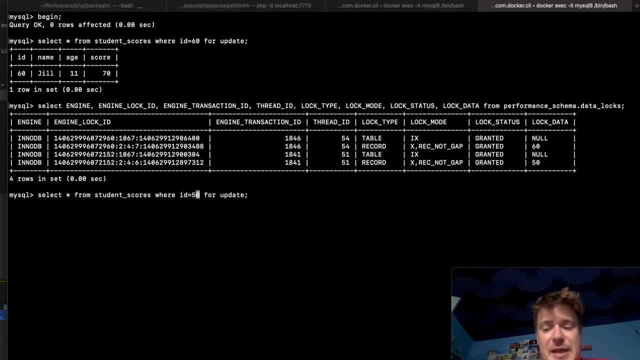 If you remember, it's the exact record that the purple transaction is holding a lock to. So, as I do it, you see it's begun to hang, because now the black session is waiting for the purple session to release the lock on the record. 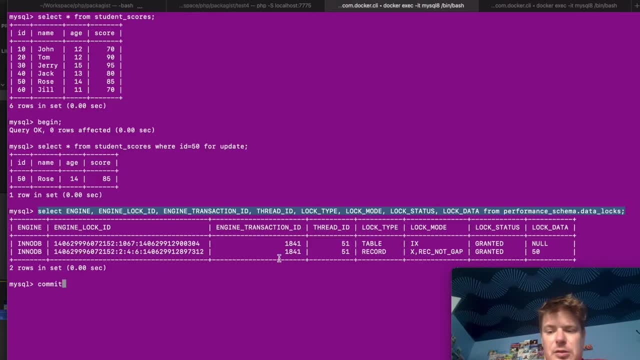 So let's jump back to the purple session. If I finish this transaction now by typing this query, I will let the black transaction proceed, but that's not what I want, because what I want is a deadlock. If you remember, the black transaction is holding a lock on the record. 60. 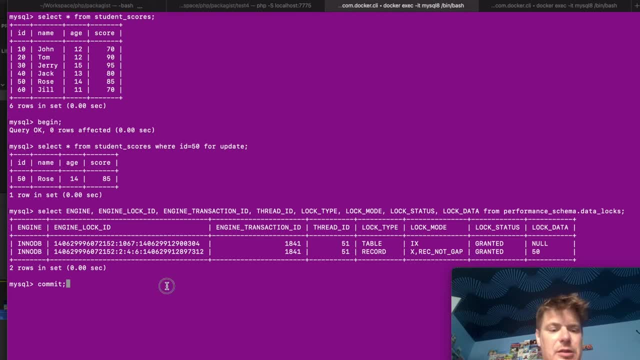 and trying to get a lock on the record 50. So what will happen if we try and put a lock on the record 60 in the purple transaction? Oops, it's a deadlock. And if we go back to the black transaction, we can see that it was able to proceed. 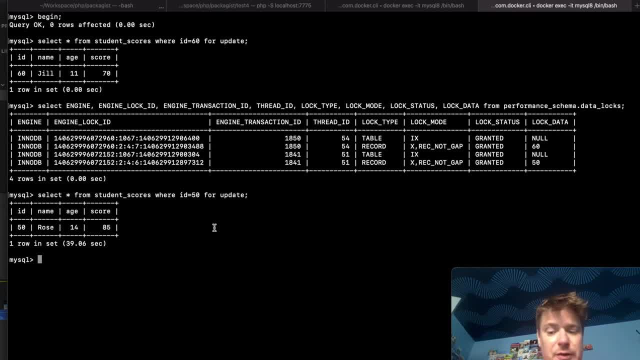 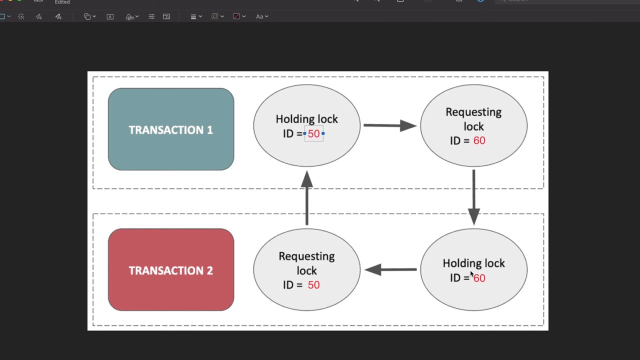 because the purple transaction was aborted and all its locks were released. In conclusion, I want to show you a picture that perfectly depicts the situation we just tried to reproduce. As you can see, transaction 1 is holding a lock on 50,, while transaction 2 is holding a lock on 60..